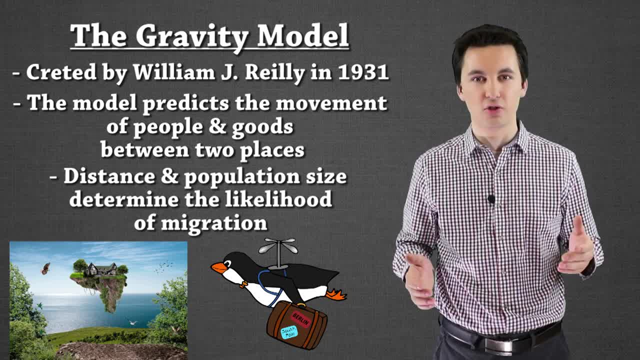 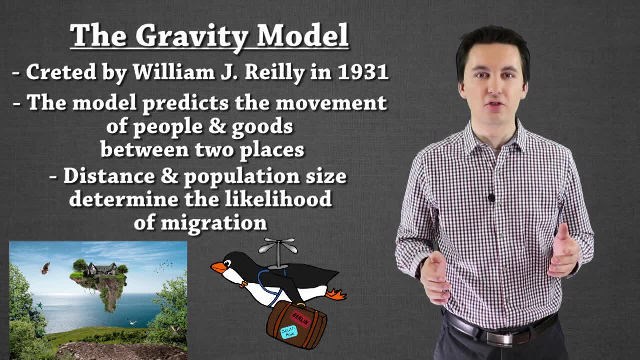 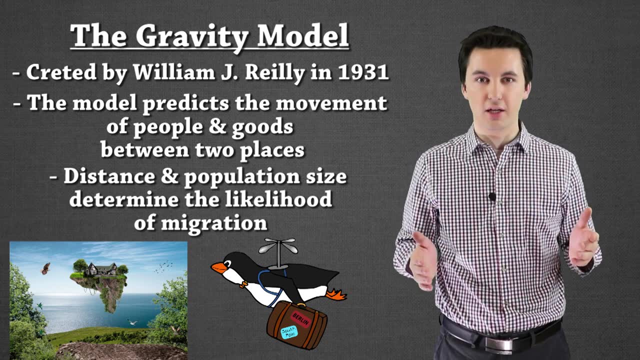 going to have less money, less people, less businesses and services, And it will attract less people then. So this concept is important to understand. The other part of this is going to be the distance between. This is actually going to connect back to distance decay: The further something away is, the less it's. 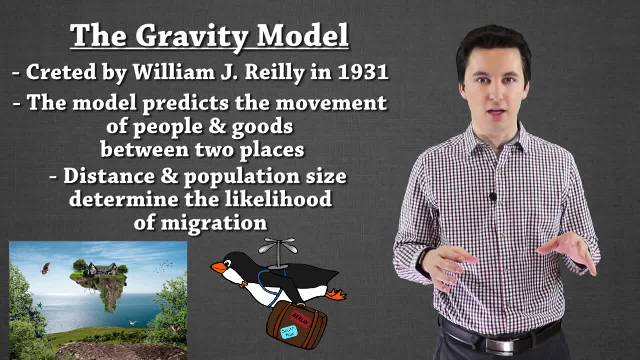 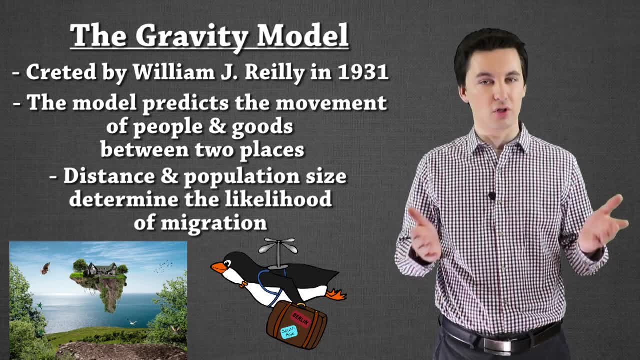 going to interact. All these concepts are important to understand. So what we're going to do right now is actually get into the formula, because we can actually use this formula to better understand exactly the likelihood of interaction between two locations. And this is the important formula for. 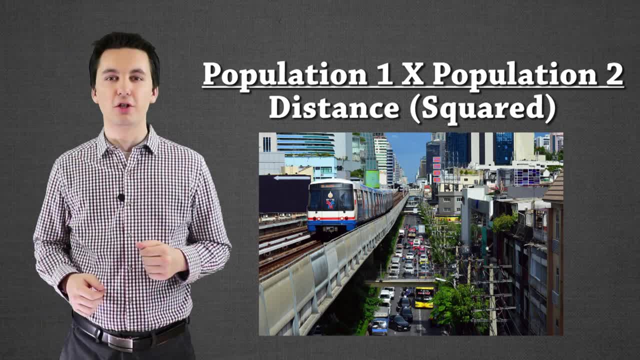 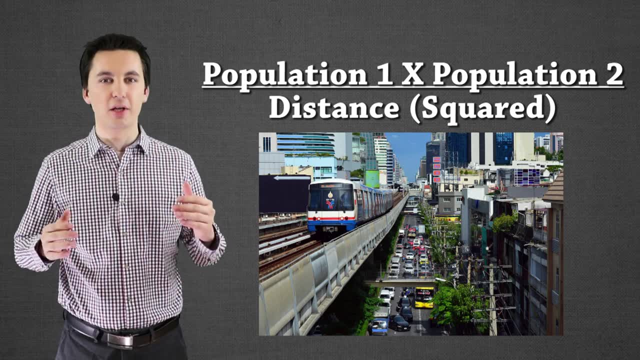 this video for the gravity model. This is the formula that we're going to use for the gravity model. We're going to take the population of city one times the population of city 2 and divide it by distance. squared Now, the distance is the distance between: 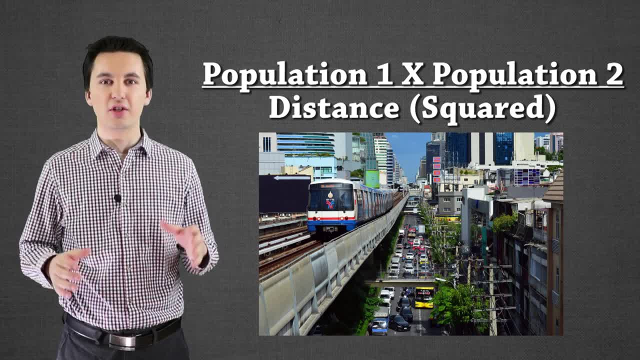 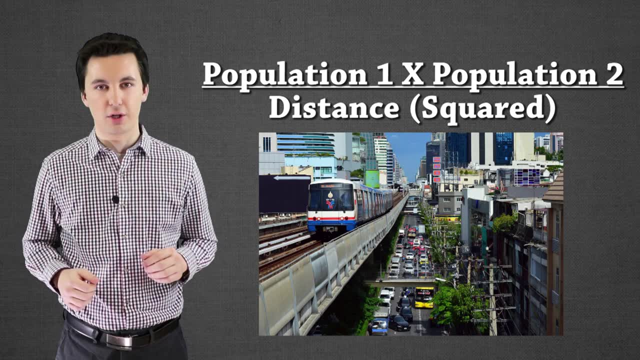 these two cities. Now, what this is showing us is the likelihood of interaction between the two cities. The larger the population of the two cities, the more they will interact, and the closer they are, the more they'll interact as well. Now, that doesn't mean that if two cities are far apart, that 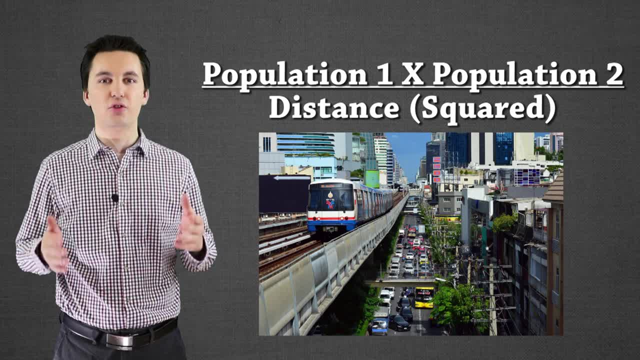 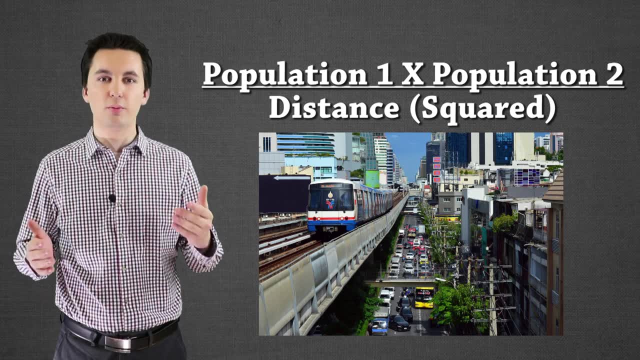 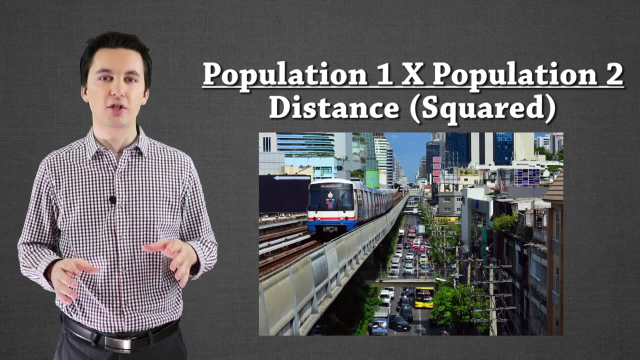 they won't actually be able to interact a lot. Actually, what we see is really large cities that are located around the world have a higher percentage chance of interacting, because when people move, they're normally going to go to areas with opportunities and those happen in larger cities. So that's important to. 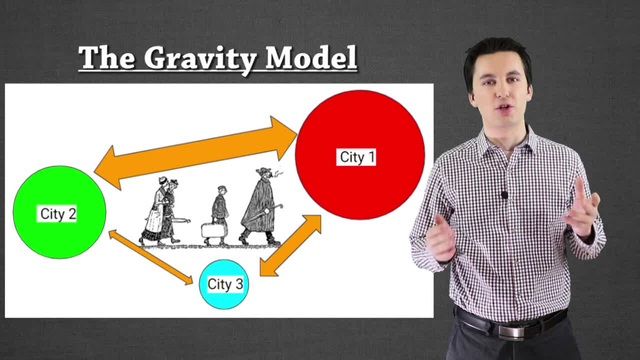 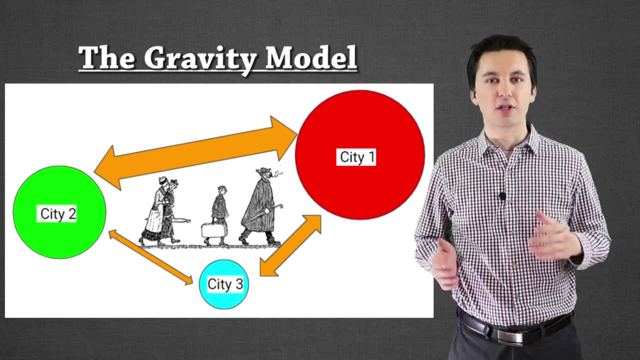 understand. On the screen here you can see actually an illustration of the gravity model. Notice how we have three different circles. The circles are different cities. The size of the circle connects to actually the population size. Now we have arrows going between these circles. 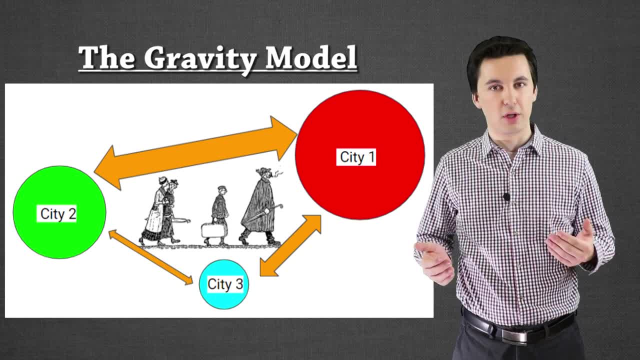 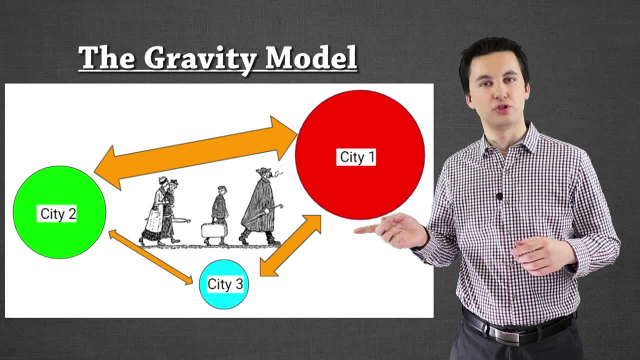 The arrows are going between these circles, The arrows are going between the two cities. Notice how those are showing us actually the interaction between the two. The larger that arrow is, the more they're going to interact. Notice how circle one and circle two are larger and they actually are interacting more with 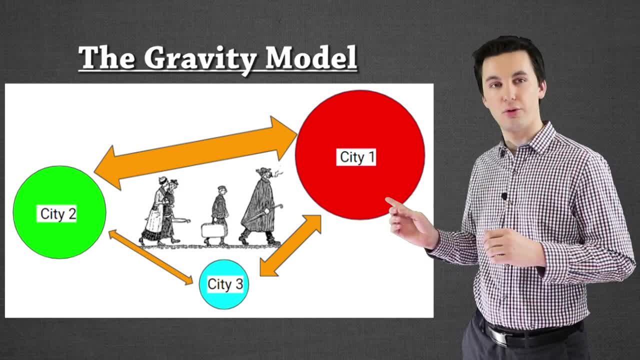 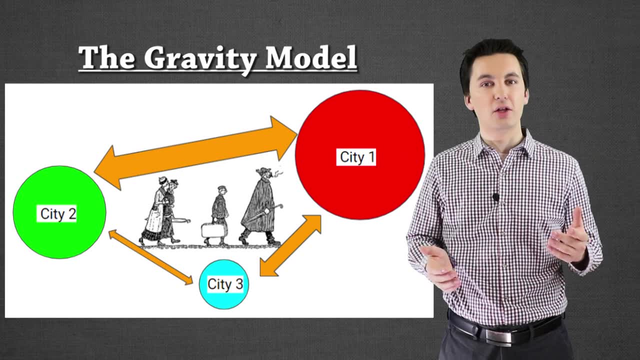 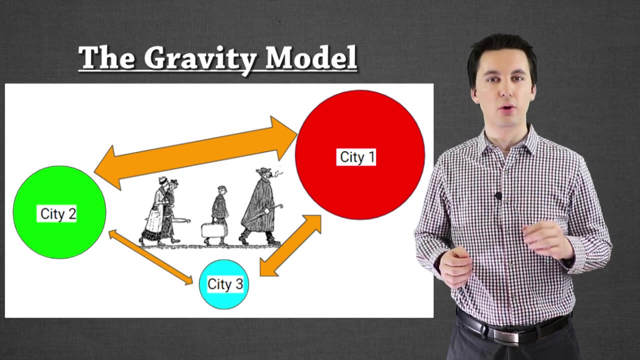 each other. Notice, then, how a circle two and three actually don't interact a lot, even though they're closer than circles two and one. That's because of the distance and also because circle three is smaller. However, circle three is closer to the large circle one, and so they also interact more frequently than 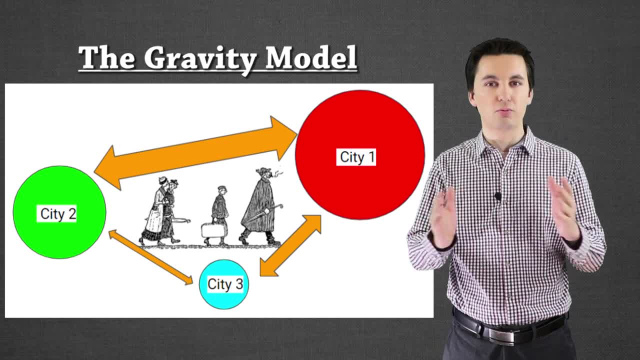 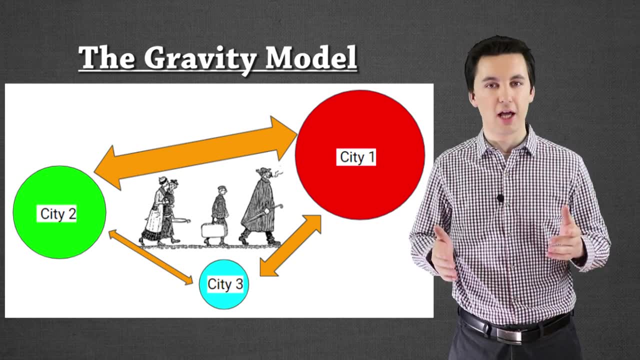 circle three and two. Now we can see this visually and really what it's just coming down to is: if you're closer to a city, you're going to interact with them more. If that city is larger, you're going to interact with it more Again. 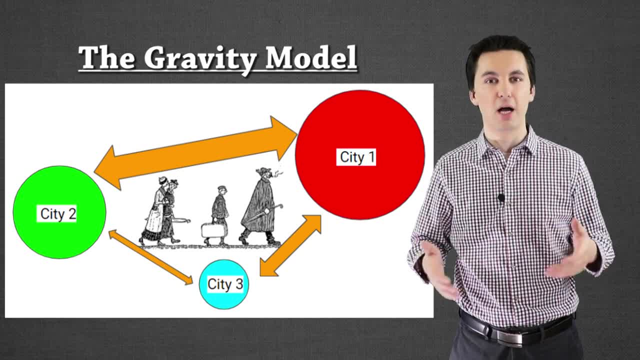 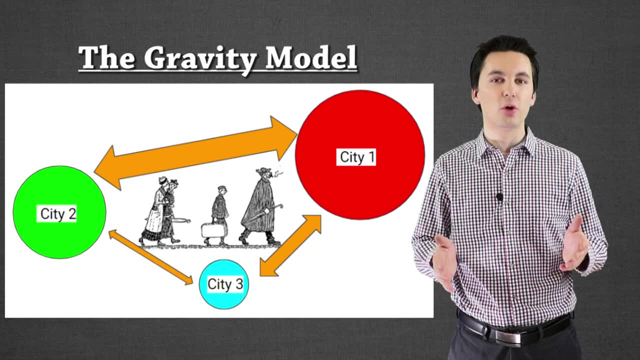 because of the opportunity, the services, the different amount of wealth and people that are located there. That's the concept. That's really all this model is saying: different migration patterns. it can show us where trade is going to happen or where businesses. 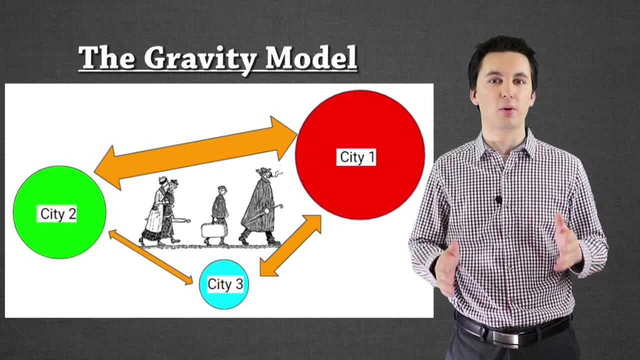 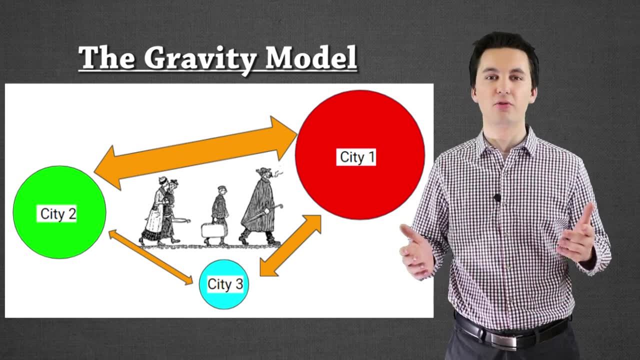 might even relocate to, And the model is just showing that And it's important for us to understand it. So, while this can get confusing, we just have to break it down And hopefully this is helping. Now on the screen, right now, I have the different assumptions that this model makes in. 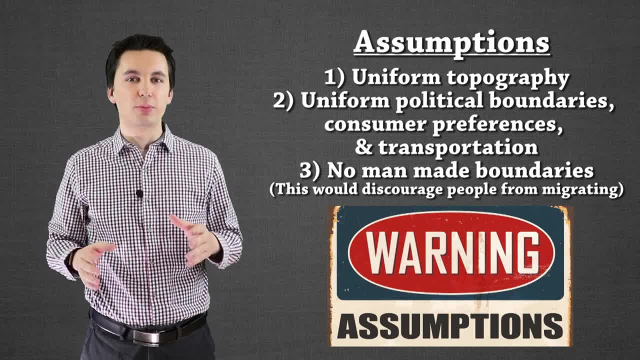 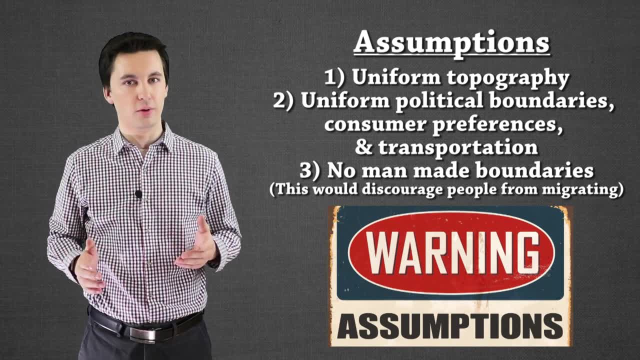 order for it to fully work. Now, I'm not going to read through them all, because I'm going to actually explain what's going on with these, So make sure to take notes on these. One of the things that we can see here is that these assumptions are not necessarily true, And in 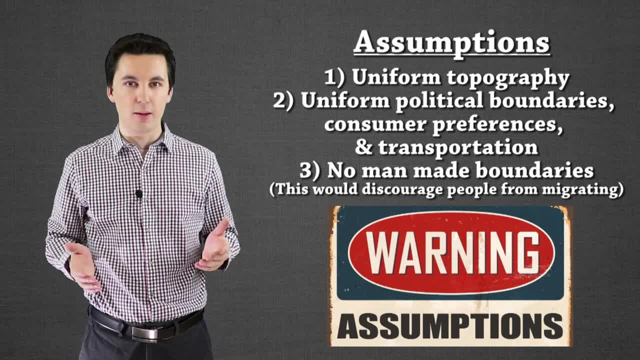 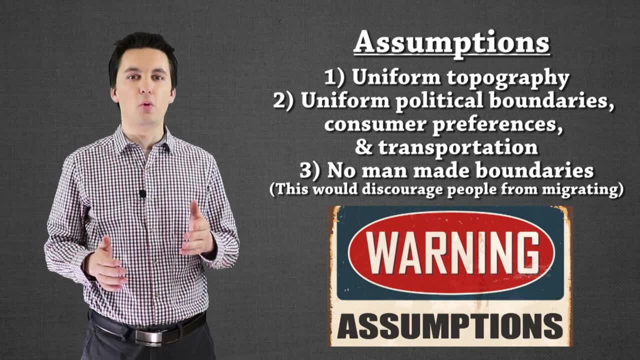 fact, the gravity model can struggle a little bit more current day because of changes in transportation and technology. People travel now for a variety of reasons. Sometimes people want to see parts of the world, Sometimes they want to visit family that are located in smaller towns or 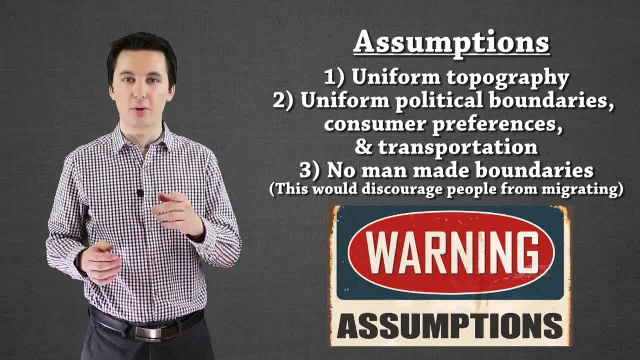 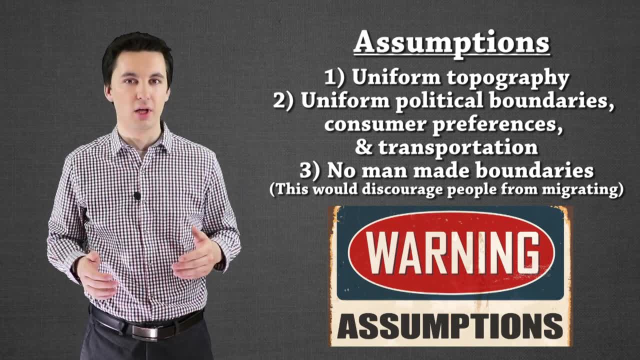 cities And sometimes they want to relocate and actually, where we're having counter-urbanization, occur away from larger populations. All of these would actually go against the gravity model. So we're going to take a look at some of these assumptions And we're going to take a look at 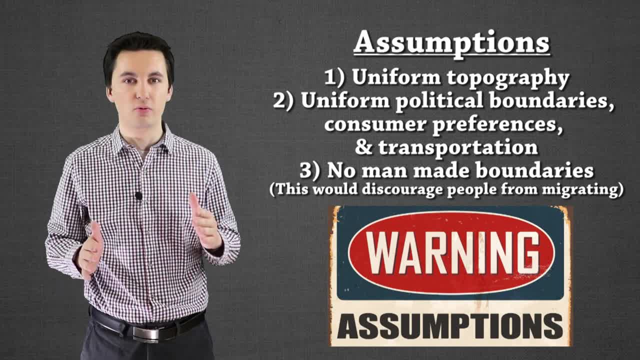 these assumptions And we're going to take a look at some of these assumptions And we're going to. The gravity model is not perfect. It's not showing exactly where movement is going to happen. It's more just showing us the chance of interactions occurring And again, that's important to